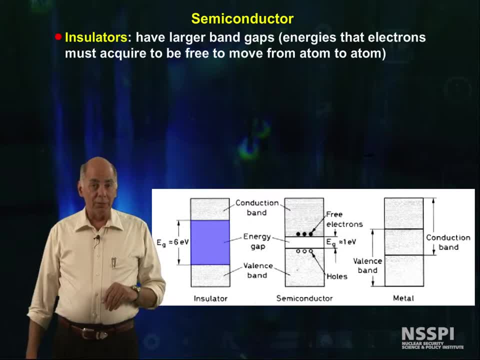 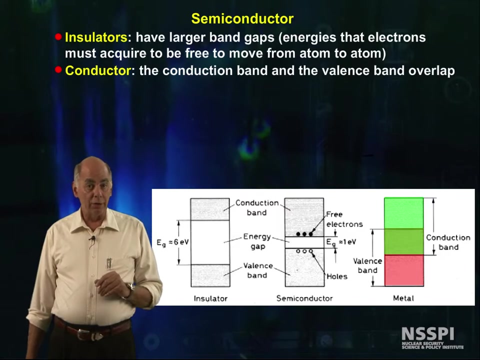 At room temperature. if the valence band is separated from the electron volts, thermal agitation caused by thermal energies cannot promote these electrons up to the conduction band. These materials are insulators. They neither conduct electricity nor heat very well. Examples are glass, ceramics, wood. You get the idea. There are some materials, almost all metals, for example- that the conduction band and the valence band overlap. 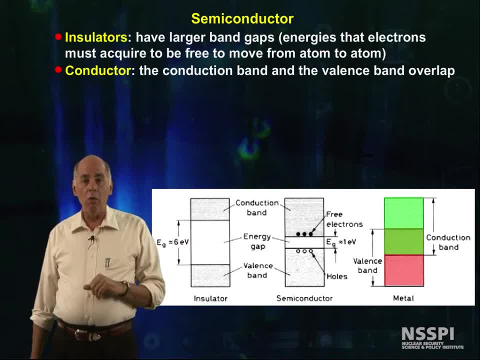 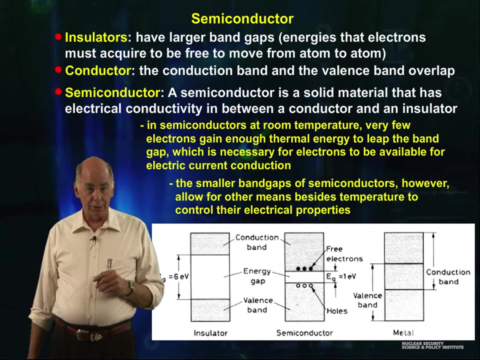 As shown here. This means that there are always free electrons that can move from atom to atom easily. These materials are good conductors of electricity and good conductors of heat. Examples would be aluminum, copper, silver and gold. There is also a strange group of actors that are called semiconductors. 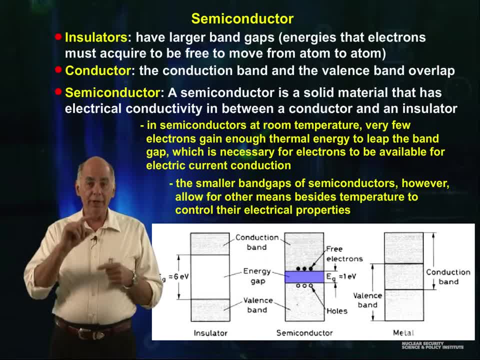 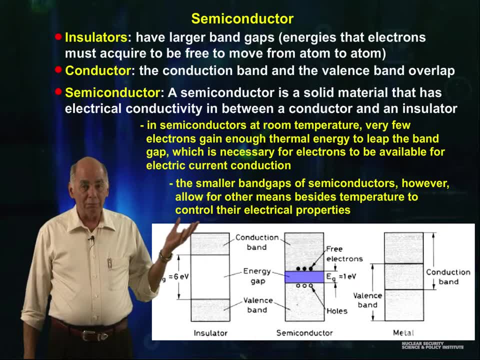 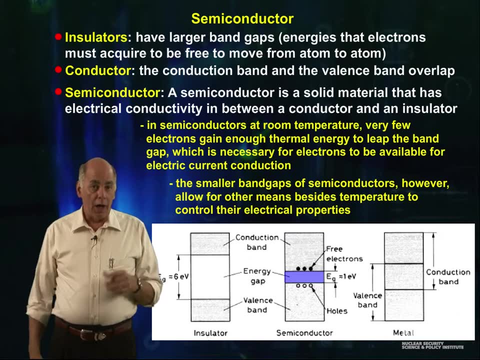 in which the valence band and the conduction bands are separated by about one electron. This is called the electron volt. Thermal energies can kick electrons up into this conduction band, but it's rare, And these promoted electrons fall back into the valence band fairly quickly. 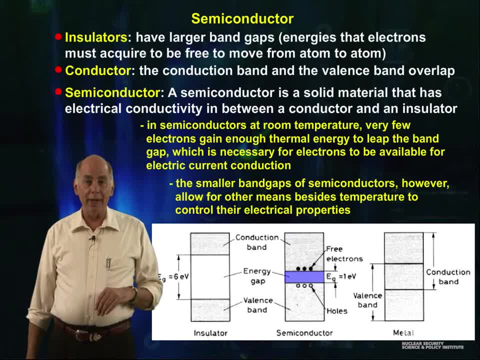 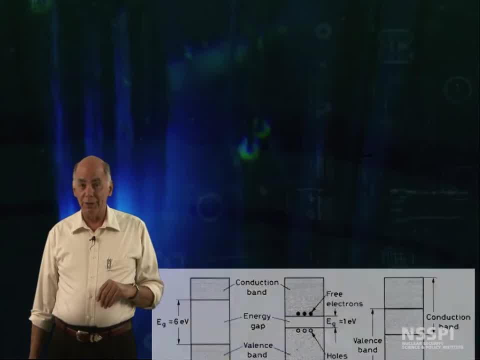 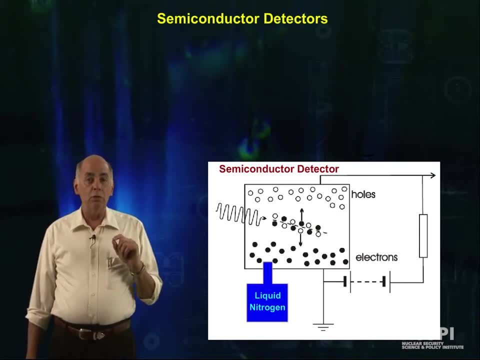 Other electrons are promoted and they fall back. so the conduction band is being continuously filled and continuously emptied, and so it's partially filled at best. We can exploit this narrow band gap to make a radiation detector. If we cool the semiconducting material down to liquid nitrogen temperatures, the conduction 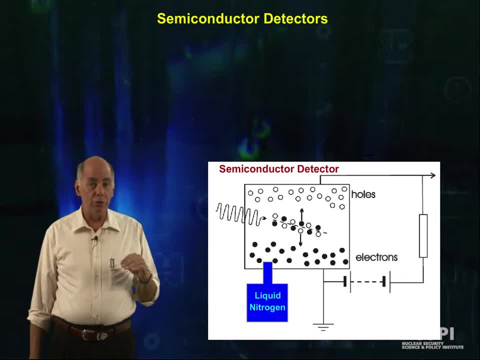 band will be empty because thermal energies are now too low to kick the electrons into the conduction band and the conduction band quickly drains of electrons. Radiation interacting in the semiconductor can promote electrons into the conduction band. An applied voltage will sweep these electrons and holes left by these missing electrons. 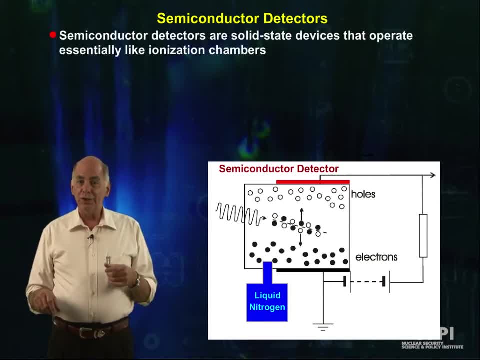 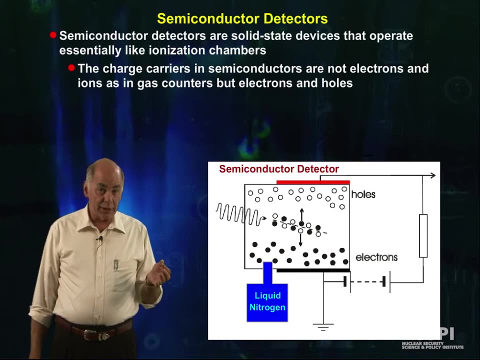 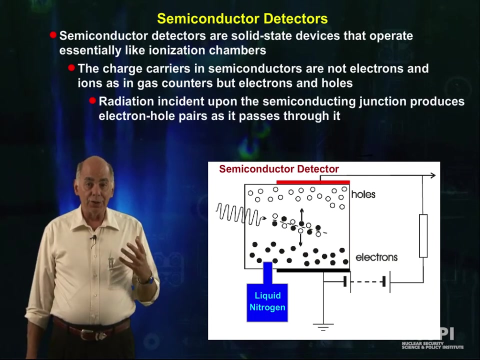 Thus, semiconductors are solid state devices that operate essentially like ionization chambers. The charge carriers in the semiconductors are not electrons and ions, as in gas counters, but electrons and holes. Radiation incident upon the semiconducting junction produces these electron-hole pairs.